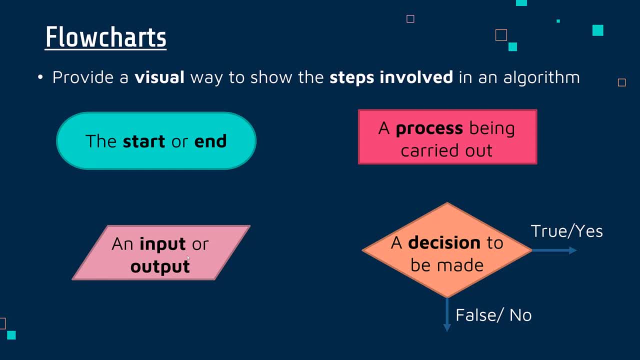 that it's either an input, so asking for something, or an output showing something. you would use a parallelogram, And maybe the most important one is a diamond, which is a decision to be made. Now, this one is where people go wrong. We should ideally only have two options, So it should really be a question which has 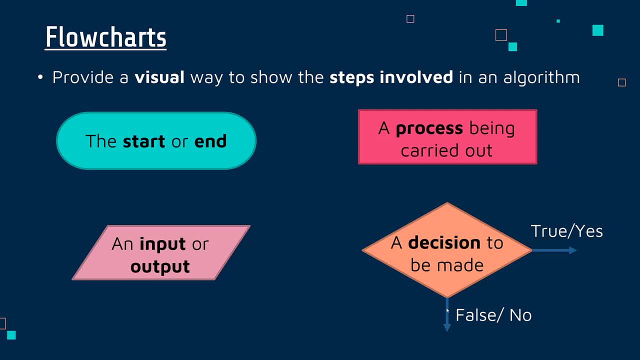 only two responses, a binary question. So, for example, if you said what is your name, that's not really suitable, but something like: are you above 180 centimeters? that would be a either yes or no answer, which would be suitable. So you've got two. 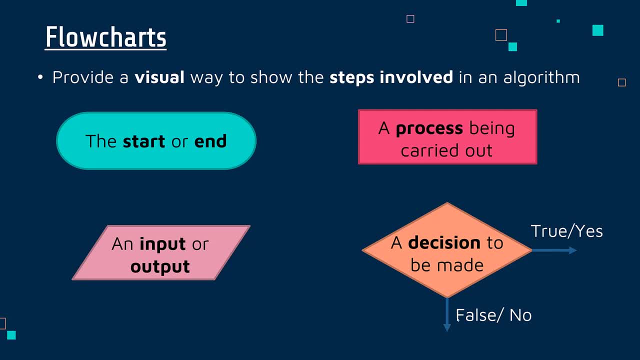 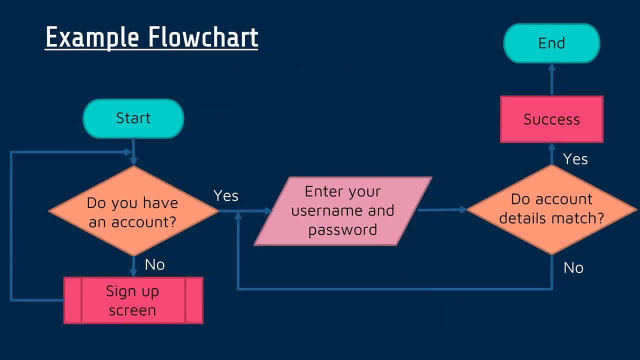 pathways coming out of it- One for true or yes, and one for false or no- And all of these are connected with arrows. So let's look at an example flowchart. This is one I made, So have a quick look at it and see if you can figure out what it's. 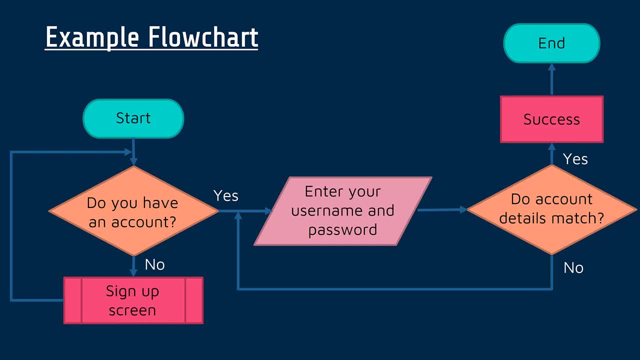 doing because a common question will be trying to interpret a flowchart So you can see we start here and we end top right. We start by asking: do you have an account? If you don't, you go to a sign up screen and it works its way back round to re-ask. 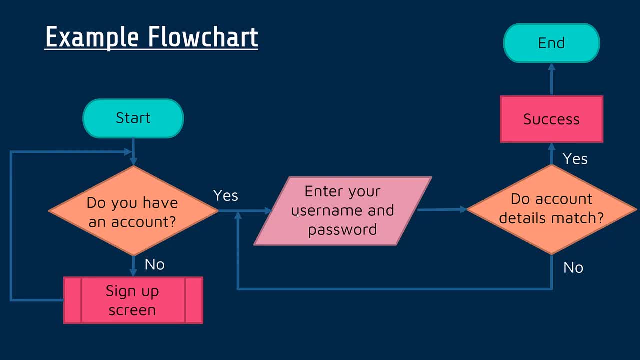 the question. If you do have an account, you're going to enter your username and password. This is an input box. You then check: do the account details match? If they don't, you loop back and re-enter the username and password. If they do match, 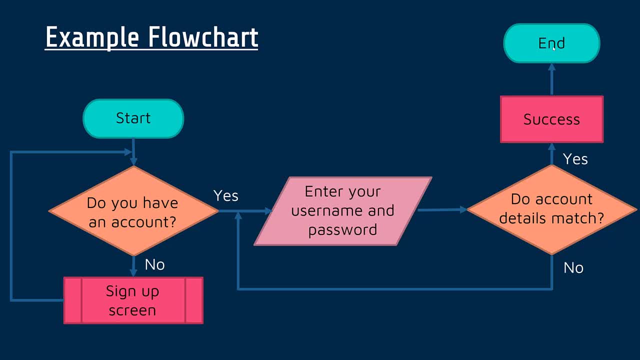 it makes a success and the program ends. So, as you probably figured out, this is for a. you know a website where you're logging in with a username and password. A fancy word is authenticating. If you are authenticating, you are, you are checking. somebody is who they say they are. Now you 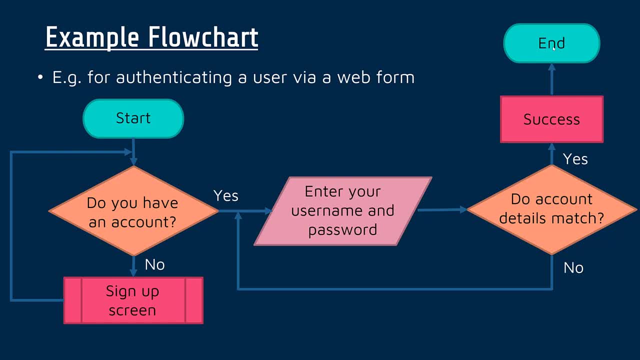 might do this flowchart a little bit differently. It's not perfect but hopefully you can see how I've used these decision shapes and they are yes or no And the arrows, hopefully, are relatively clear the direction they're following. Make sure every arrow has a an arrowhead Right. You could just do a. 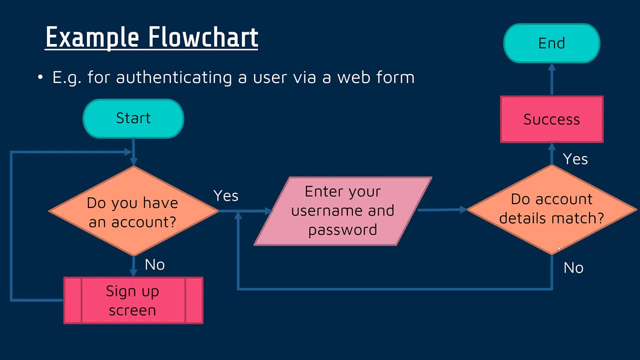 straight line, make sure it's got a direction, and it's fine to loop back, and you'll often do this. when you want to repeat something, Just make sure it rejoins at the place you want it to like here and like down here. Now this symbol.